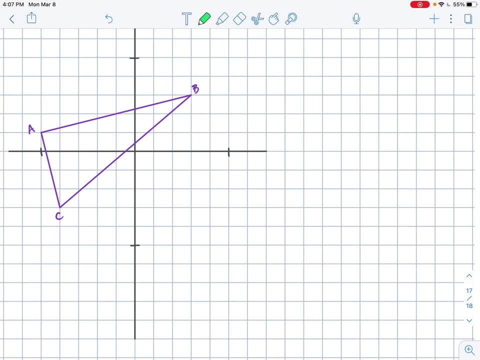 So here we have a triangle and I want us to find the area of this triangle. So I know that the formula for area of a triangle is one half times the base times the height. So usually what we've been doing in class is looking at right triangles only. So if I look at this triangle, it looks like 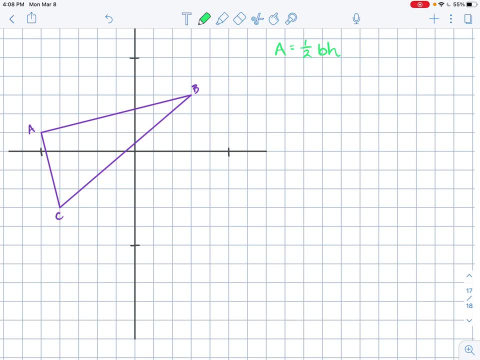 angle A might be a right angle. So to figure out if that's true, I'm going to find the slope of segment AB and segment AC. So for segment AC that's down 4, right 1.. So the slope of segment AC is negative 4 over 1.. For AB: 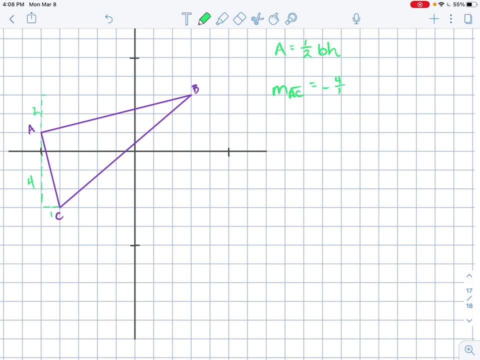 that's up 2, right 8.. So the slope of segment AB is positive 2 over 8.. Now 2 over 8 can simplify to be 1 over 4.. So these are my slopes: negative 4 over 1 and positive 1 over 4.. 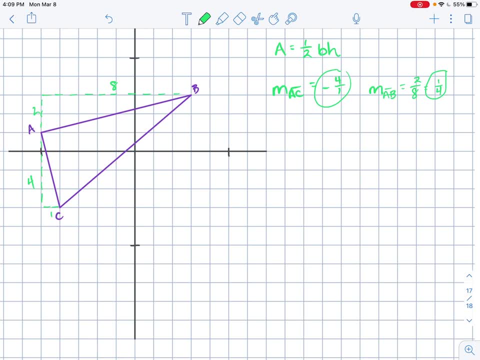 And I notice those are opposite reciprocals. So because those slopes are opposite reciprocals, that means that these sides, AB and AC, are perpendicular, which tells us that angle A is in fact a right angle. This is great, because in a right triangle, 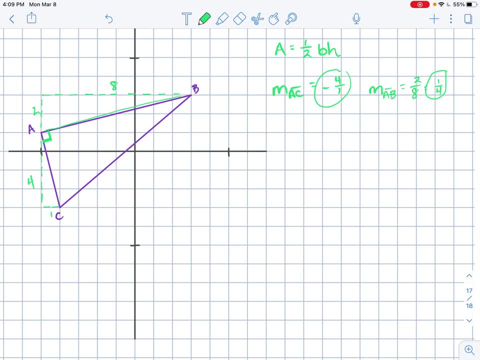 the two legs. so AB and AC will be the base and the height when I plug in. So let's go ahead and do that. I need to figure out the length of the base and the height, So I'm going to start with the length of AC. Again, the rise and run were 4 and 1.. 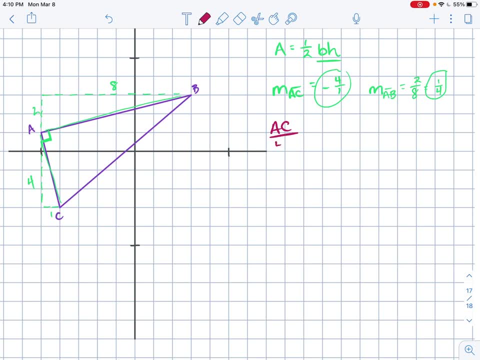 So I'm going to plug that into the Pythagorean theorem. So 4 squared plus 1 squared equals c squared. 4 squared is 16. 1 squared is 1. That's still equal to c squared. When I add those together, it's 17.. So AC is radical 17.. Now let's look at AB. 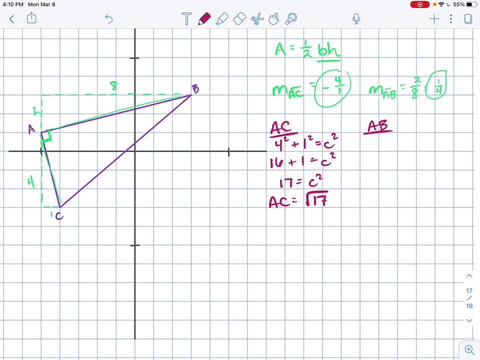 So in the Pythagorean theorem I'm going to plug in for A and B, 2 and 1.. So I'm going to plug in for B and B, 2 and 1.. So I'm going to plug in for A and B, 2 and 1.. 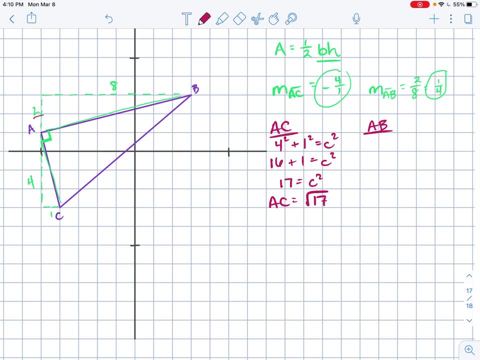 So in the Pythagorean theorem I'm going to plug in for A and B, 2 and 1.. 8- again that came from the rise and run. so 2 squared plus 8 squared equals C squared. so that's 4 plus 64. so 68 is equal to C squared. that means that a, B 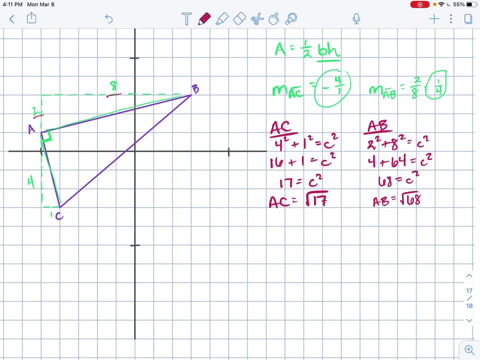 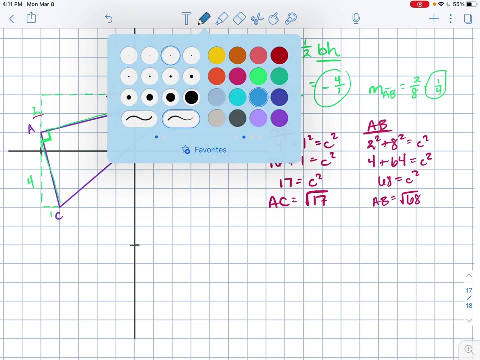 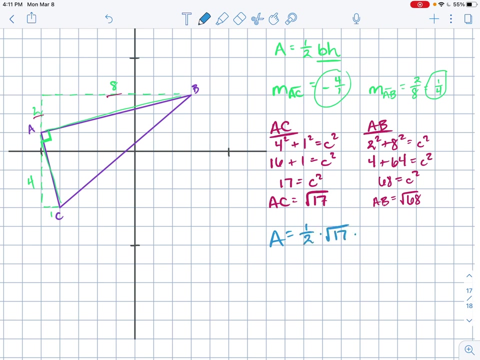 is equal to radical 68. okay, so I'm going to use radical 17 as my base and radical 68 as my height. it really doesn't matter. which is which, since I'm just multiplying so, the area will be 1 half times radical 17 times radical 68. 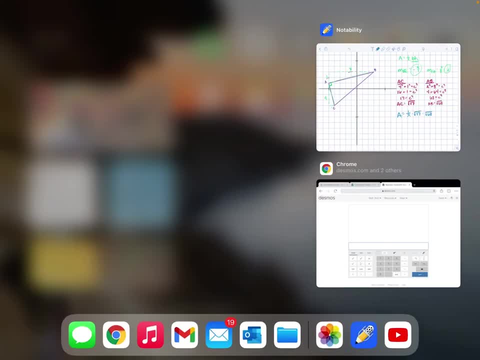 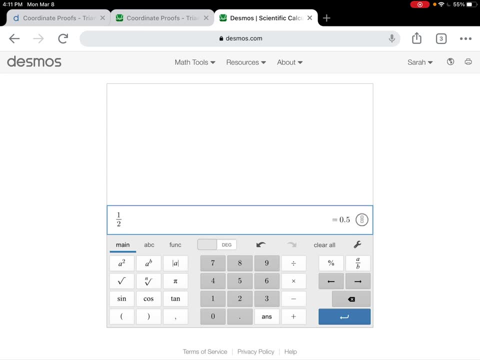 and I'm just gonna type all of that into the Desmos scientific calculator. so one half after I type in one half, I need to make sure I move my cursor over so I'm not in the denominator anymore. times radical 17. again I need to move my cursor over so I'm not within the 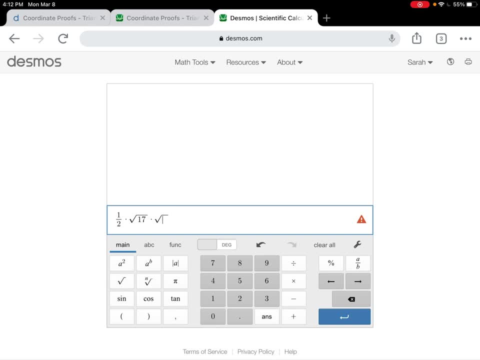 radical anymore, times radical 68 and that gives me 17. so the area of this triangle,